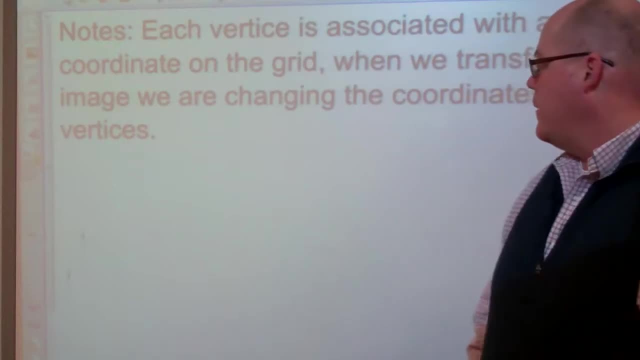 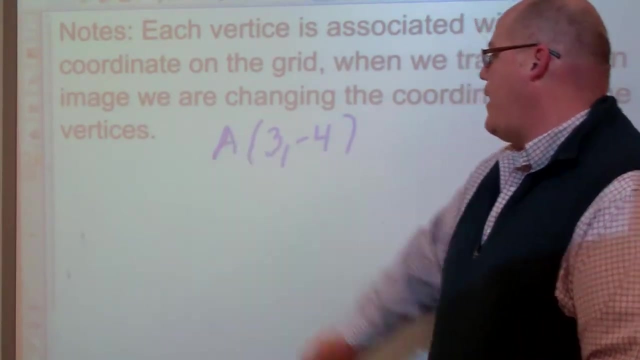 Again, Mr Collins, if you could pause this to make sure they get this in their notes for me, Alright. So let's say three negative four. Let's say that's point A. So the coordinates for point A is x is 3 and y is negative 4.. 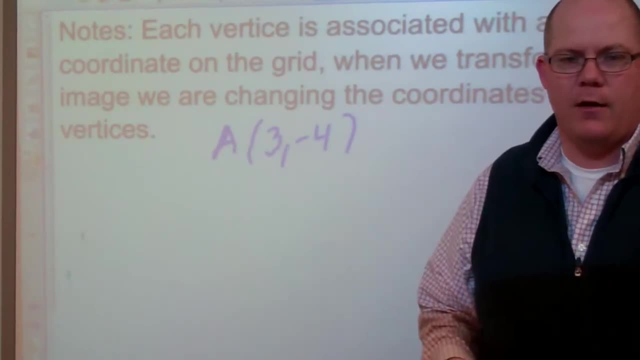 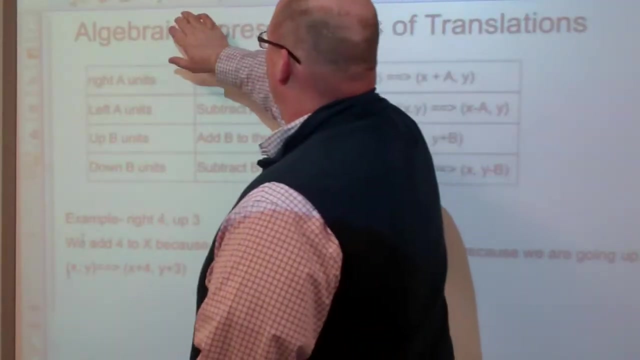 And you can translate that: rotate it or flip it and we'll talk about: I'm sorry or yeah, flip, reflect it. So, Mr Collins, we're going to pause here, Mr Collins, so that they can get this in. 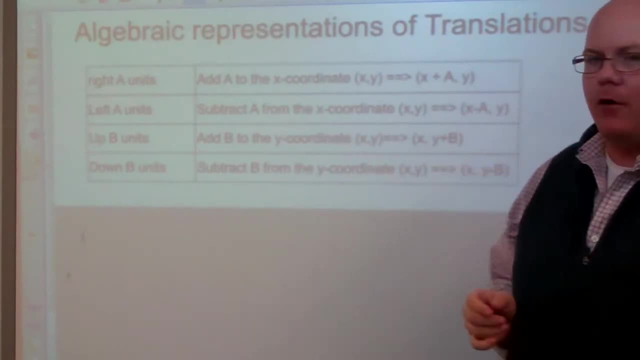 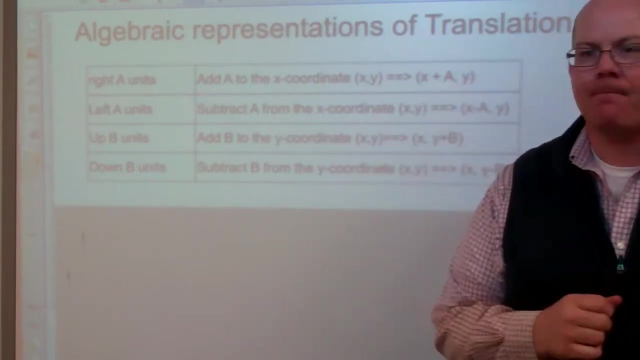 their notebook. This is Algebraic Representations and Translations. It's going to go in your notes section, so make sure you have the title and then draw the table or the chart. All right, welcome back. So you got that done. 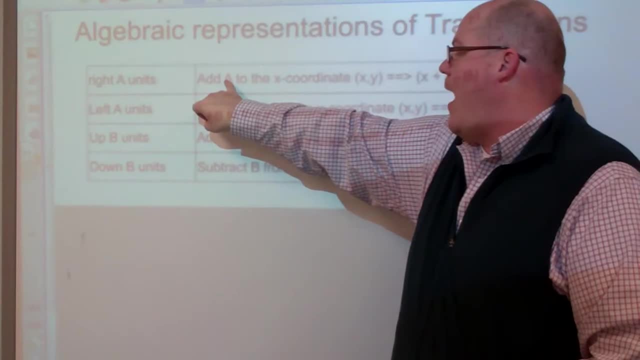 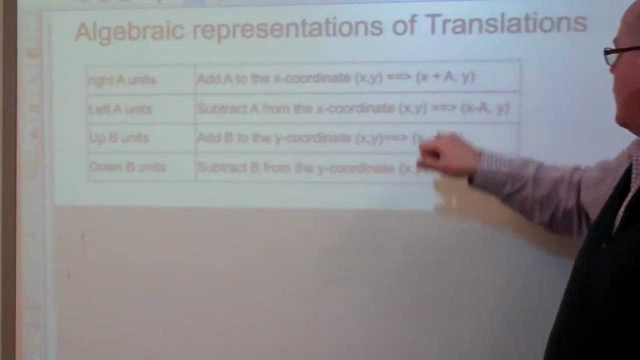 So when we move right a unit, we're going to add the value of the translation, or what we call a, to the x coordinate. So if we're going right- 3 units, we would add 3 to x because we're going right on the. 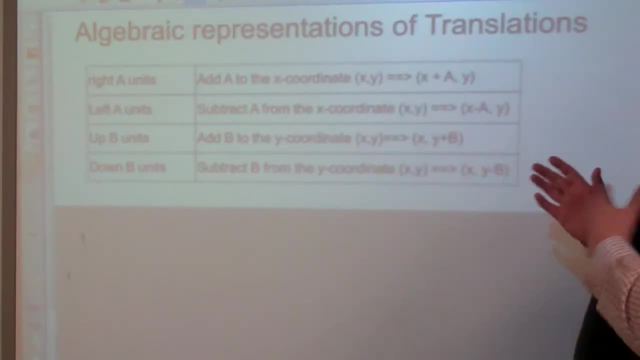 number line. The origin is 0.. We're moving to the right, so we're adding to the x value. So we have x plus a y. doesn't change. when we go right, When we go left, we're adding to the x value. 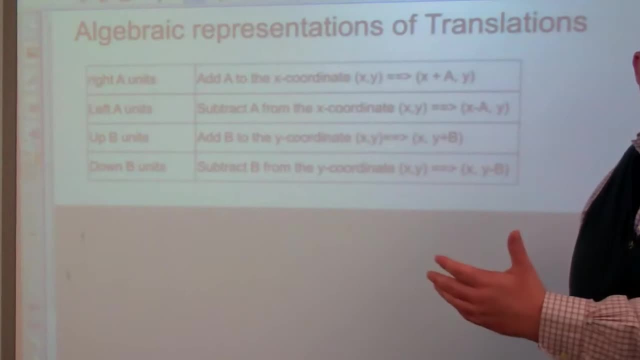 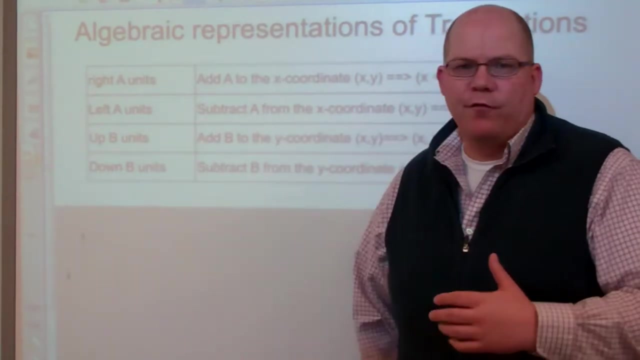 When we go left opposite, we're subtracting value and we're moving left or negative down from the origin. so we're subtracting values from that. When we go up or down, we're moving along the y axis. right we're going up from the. 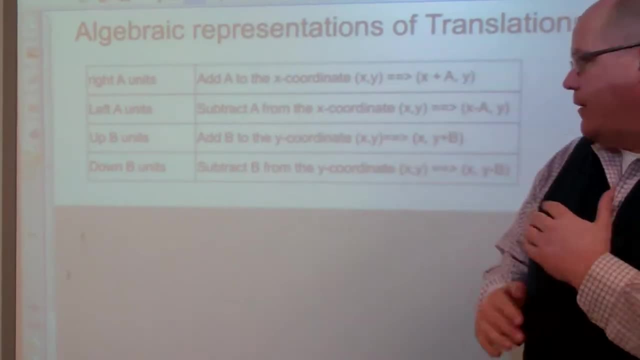 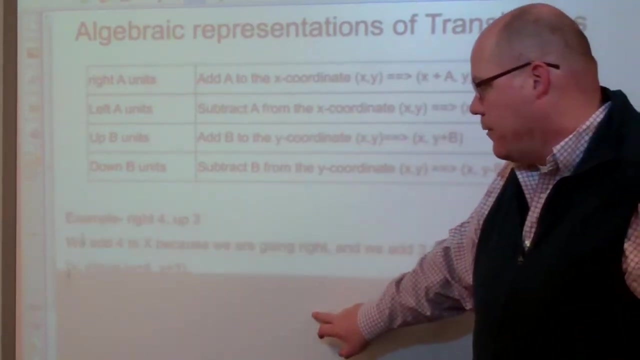 origin or down. Up is positive, down is negative. So if we go up we're adding to y, When we go down we're subtracting from y. So a quick example here: if we're going right, 4, up, 3.. 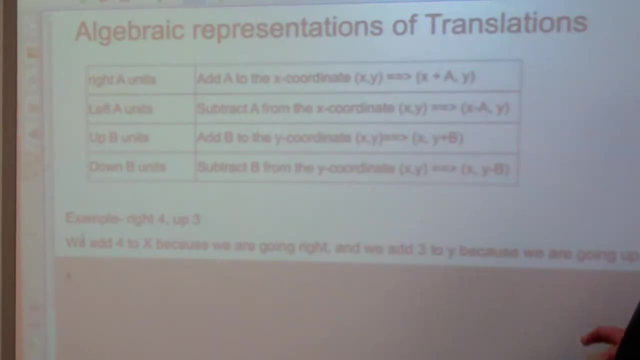 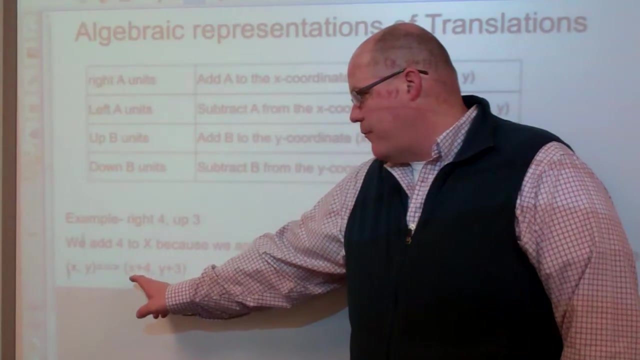 We add 4 to x Because we're going to go right and we add 3 to y because we're going up. So algebraically it would look like this: The x and y coordinate would become x plus 4, comma y plus 3.. 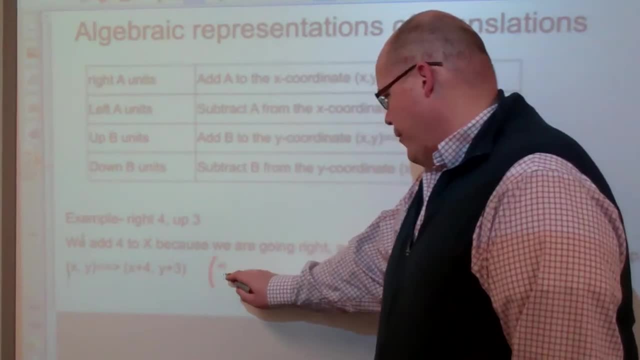 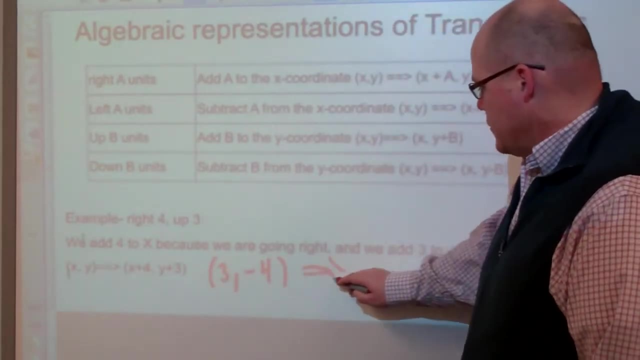 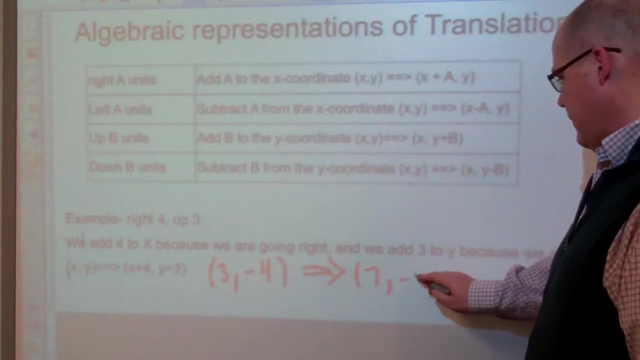 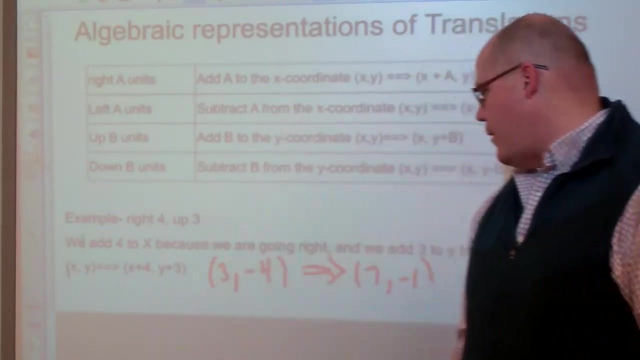 So if we had 3, negative 4,, we're adding 4 to 3.. So this becomes 7, and we're adding 3 to negative 4.. This becomes 0. This becomes negative 1.. So when we translate 4 to the right and up 3, we go from 3, negative 4, to 7, negative. 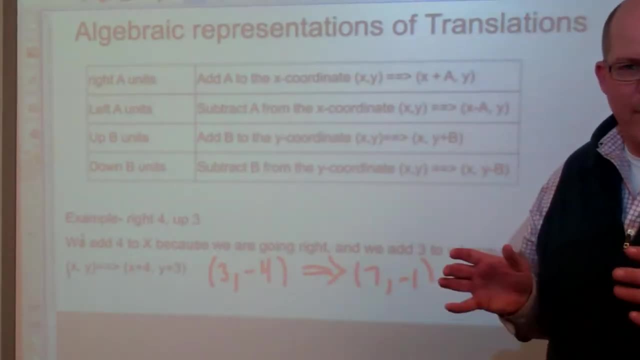 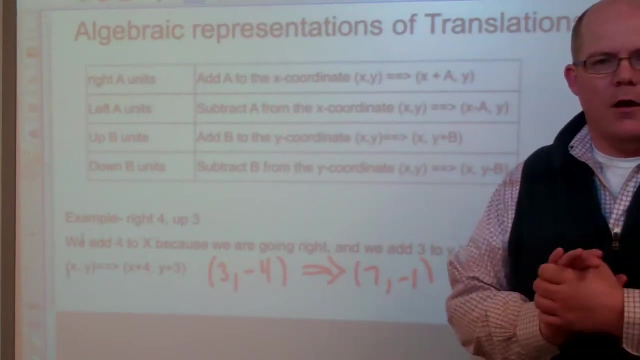 1.. Next, I'm going to have you guys do a little bit of practice. so you're going to draw the table, I'm going to give you the rule and then we're going to pause the video so that you can have time to complete the rest of the table, and then Mr Collins will go over the 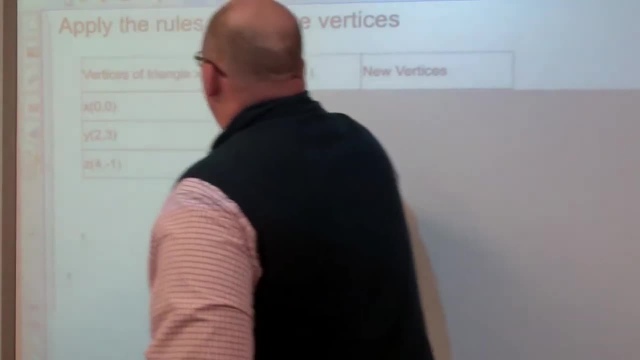 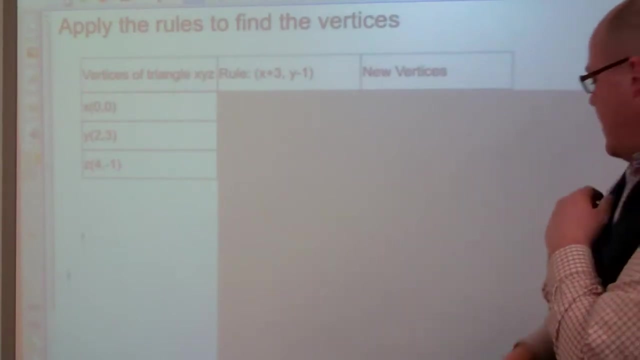 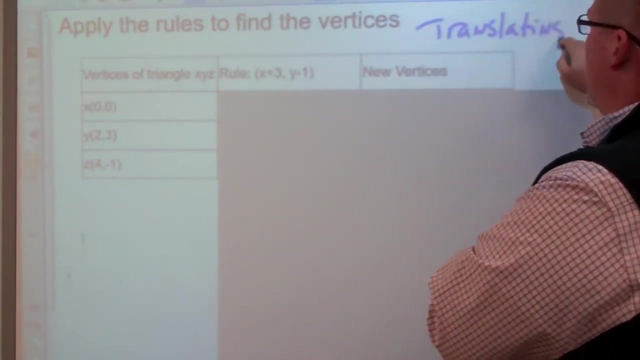 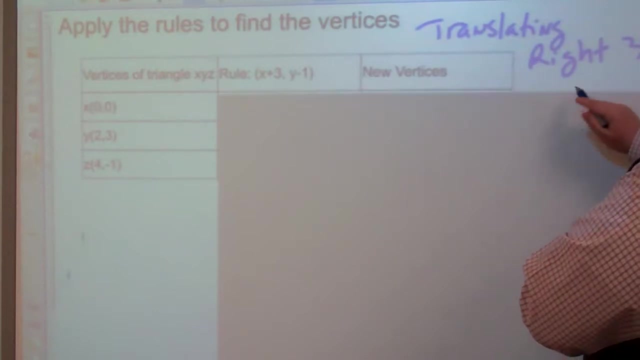 answers with you. So let's go ahead and in your notebook, let's title it: Apply the Rules to Find the Rules, And you're going to write down the vertices. We're going to be translating. Let me write this down. We're translating right 3 and down 1.. 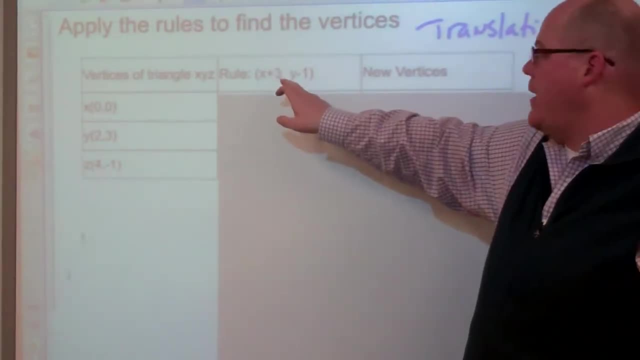 So we're translating right 3 and down 1, so you see we're adding 3 to x and subtracting 1 from y. Why don't you guys go ahead and pause here so that you can see this? You can see that we're adding 3 to x and subtracting 1 from y. 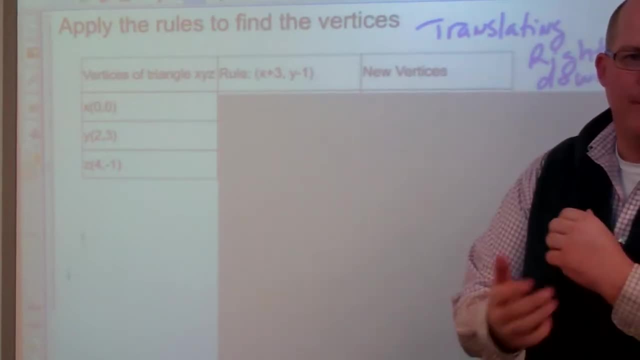 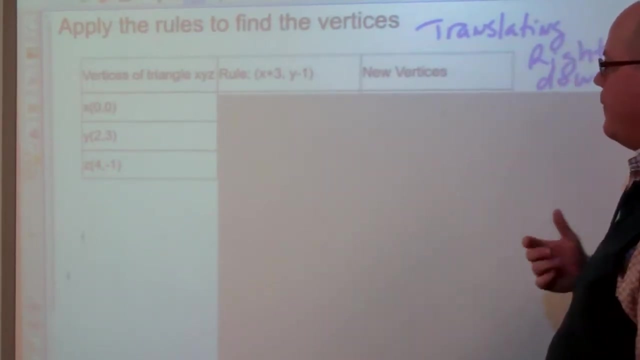 All right, So we're going to go ahead and draw the table and complete the table. All right, Great, Welcome back. So now that you have an opportunity to go ahead and apply the rules and find the new vertices, let's see how accurate you are. 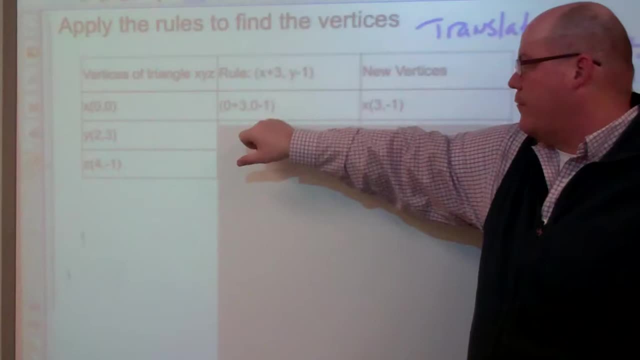 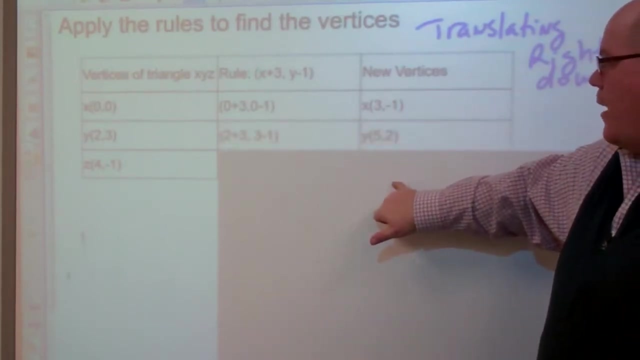 So when we add 3 to x and we subtract 1 from y, our new value, our new vertice we have x is 3, y is negative 1.. For y we add 3 to 2, subtract 1 from 3, and our new vertice is 5,2, and for z we add: 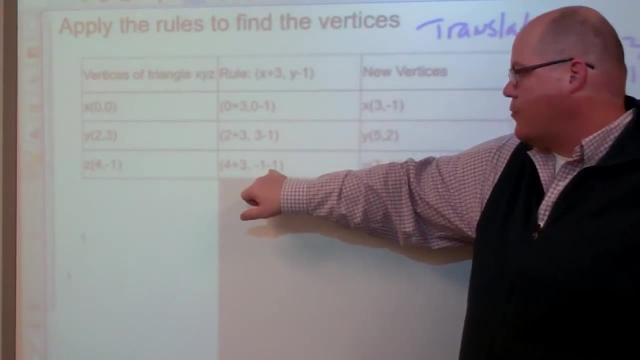 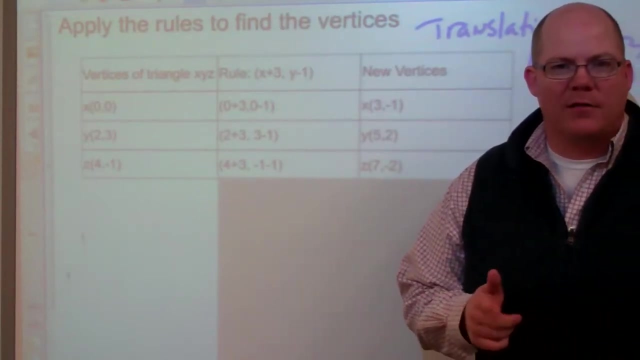 2. z We add 3 to 4 and subtract 1 from negative 1. Our new vertice is 7, negative 2. So translation is pretty simple: We're adding or subtracting to the x and y value, depending on whether or not. 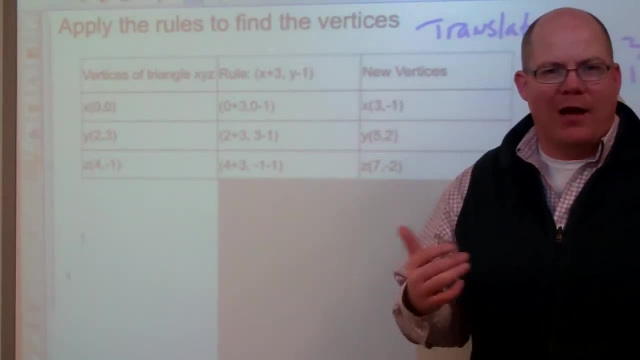 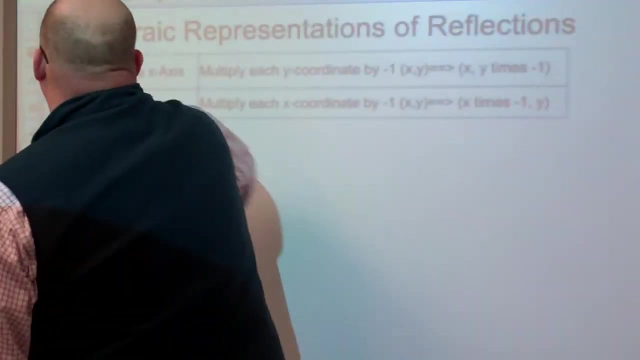 we're translating right, left, up and down. We're just adding or subtracting that value to each of the x and y values for all of the vertices of the object or the shape. Let's take a look now at representations of reflection. So again, I'll just pause here for a sec. Pause the video. so. 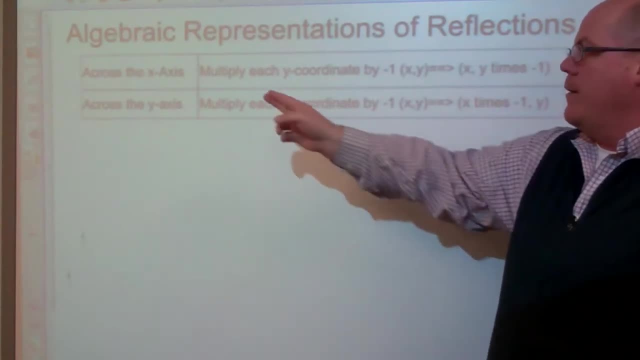 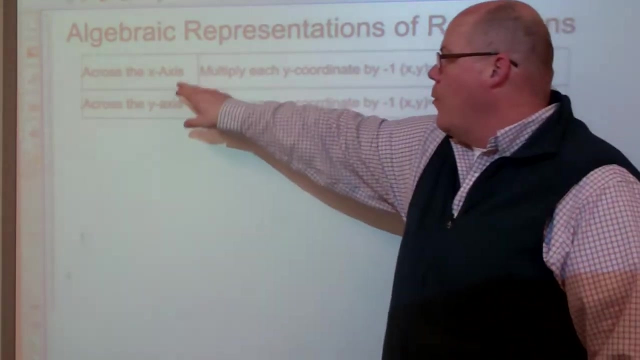 that you guys can copy this down in your notes. Make sure you get the table and write down the rules for the notes. All right, great, Now that you got that done, let's quickly just talk about it. When we're reflecting, all we're doing is we're flipping across the x or we're flipping 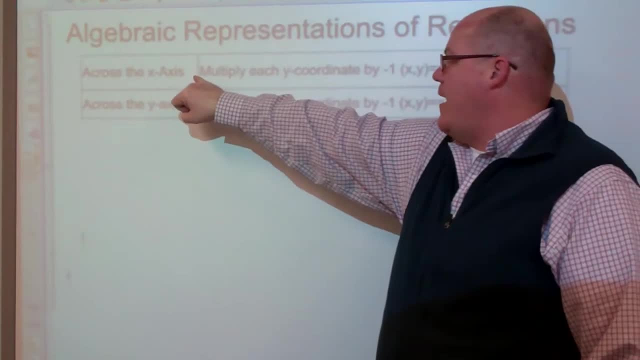 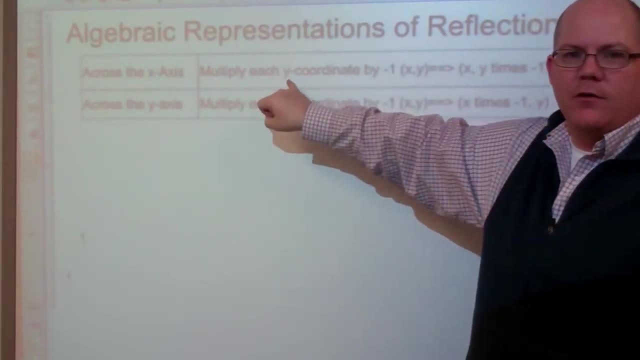 across the y-axis. When we cross the x-axis, the x values don't change. The y values change. So what we do is we're going to multiply each of the y values in the coordinates of all four of the vertices, or three or five times the x-axis. So what we're going to do is we're going to 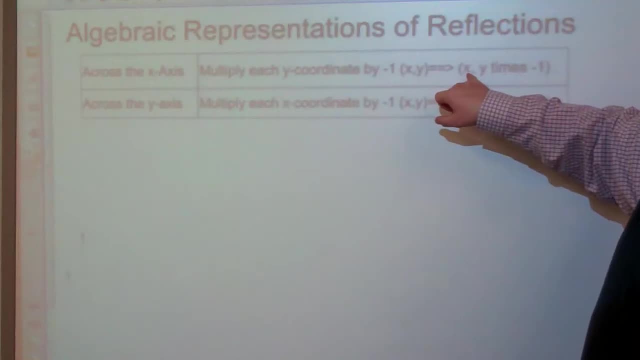 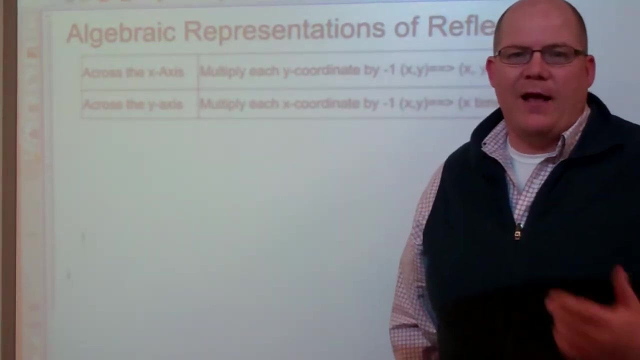 multiply each of the x-axis, or three or five times the x-axis, or three or five times the negative one. So xy becomes xy times negative one. When we do it across the y, all the y values are staying the same, but the x values are changing. So same thing. we're going to multiply negative. 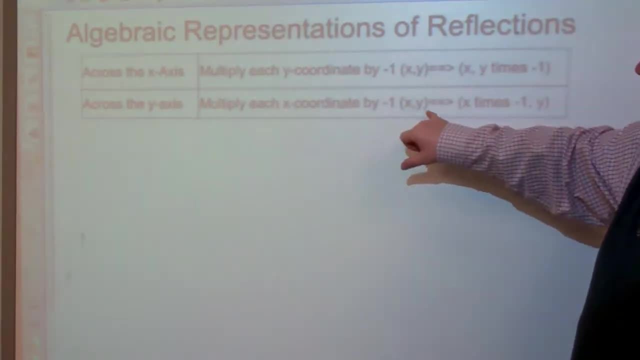 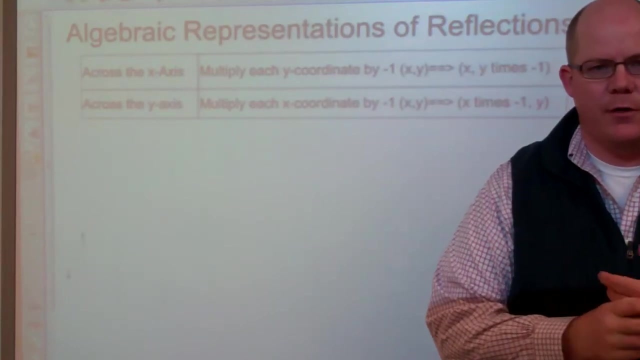 one times each of the x-coordinates. So xy becomes x times negative one and y. All right, real, real simple. Let's go ahead and look at a table and give you guys an opportunity to complete a table. So here we're going to apply the rule to the vertices We're going to apply. 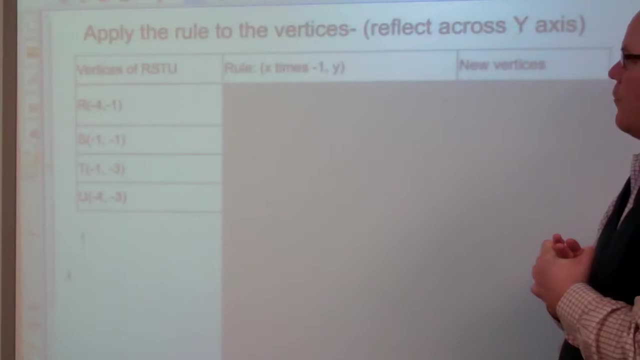 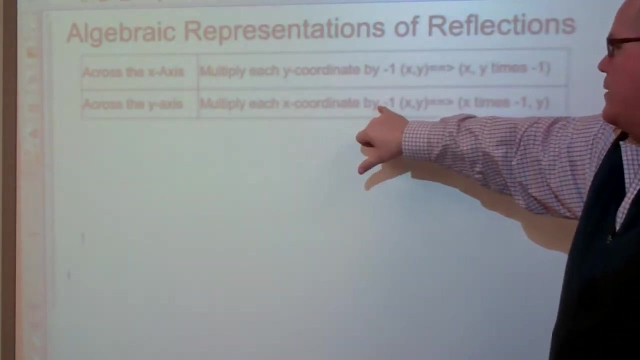 the rule to the vertices. We're going to imagine we're going to reflect across the y-axis. So remember, when we're reflecting across the y-axis, we're going to multiply each of the x-coordinates by negative one. So that's going to be our rule here. Rule x times negative one y. So if you 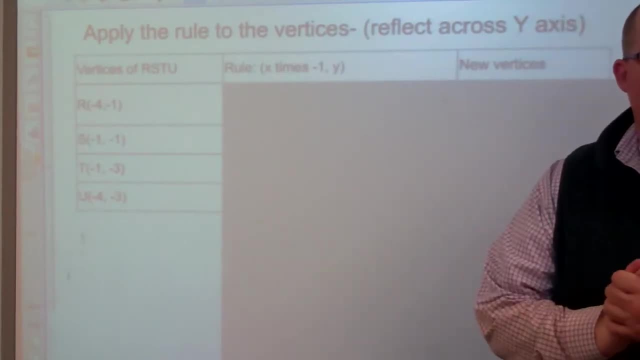 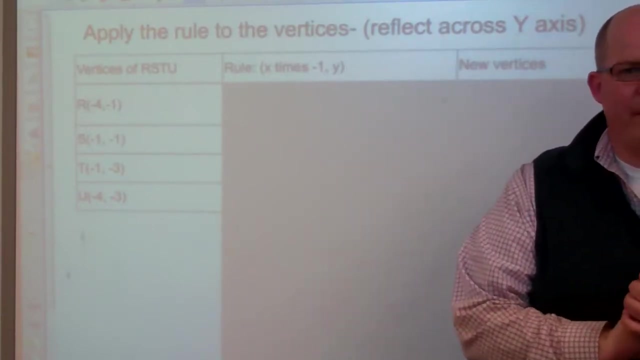 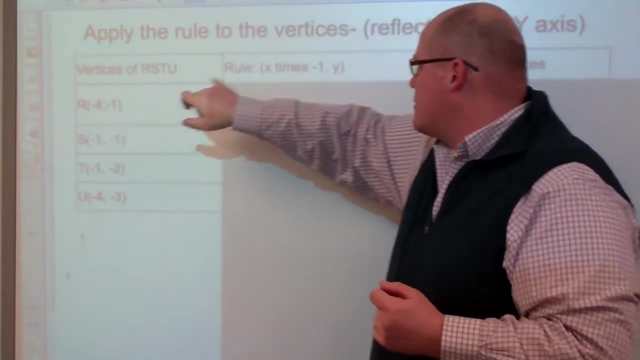 guys go ahead and copy this table down in your notes and then pause the video so that you guys have an opportunity to complete the table. Now that you have an opportunity to do that, let's quickly go over the answers. So when we multiply x times negative one and y, negative four is x, So we multiply that times. 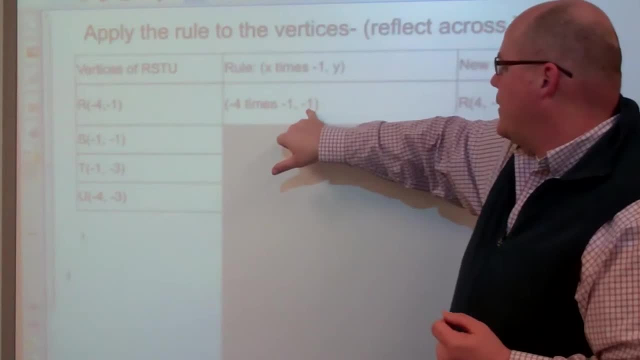 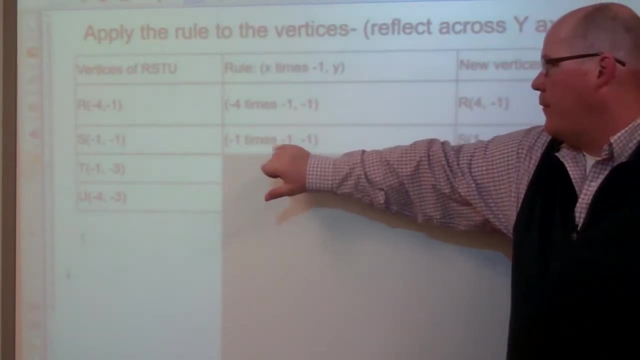 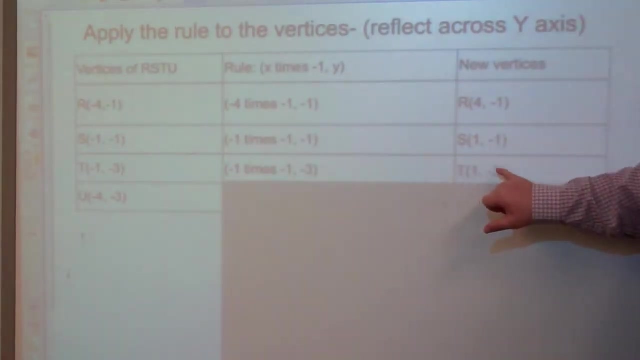 negative one. And y does not change. So our new value, our new vertices, becomes four negative one. For s follow the same rule. Our new vertices: one negative one. T. our new vertices becomes one negative three. And u. our new vertices becomes four negative three. So you. 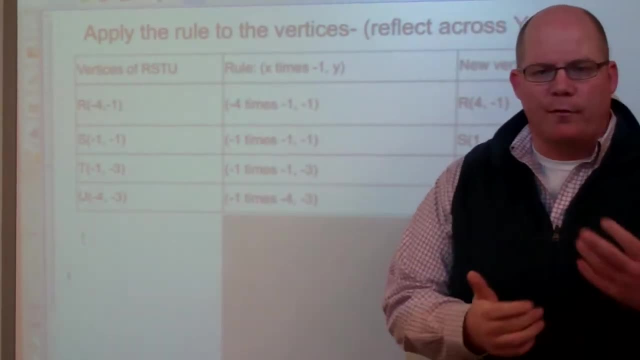 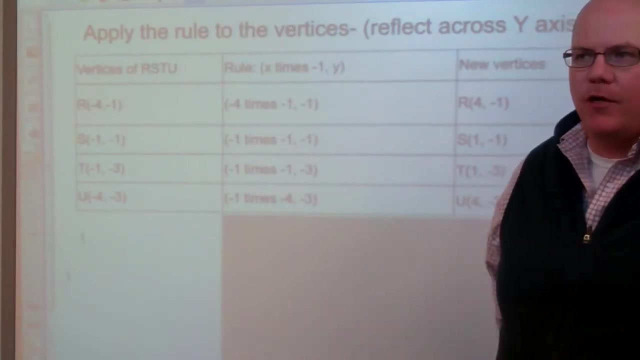 can go ahead and do that. So each of the four vertices we apply the exact same rule. The rule that we apply depends on what we're doing, So here we're reflecting across the y. So the rule is to multiply x times negative one, And y does not change. Let's do one more rotation, So we're. 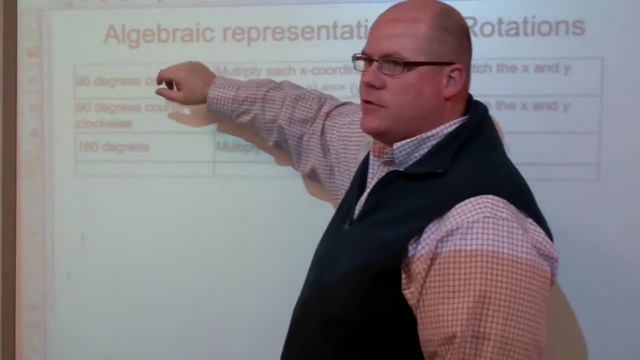 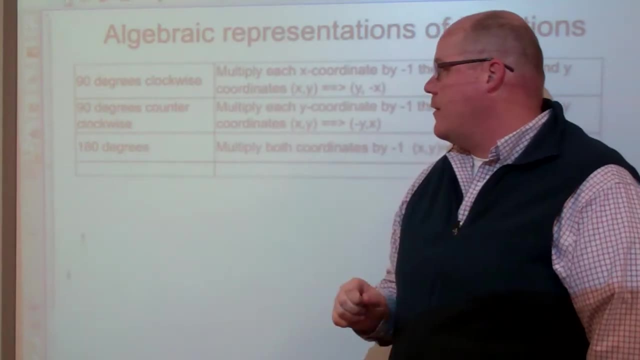 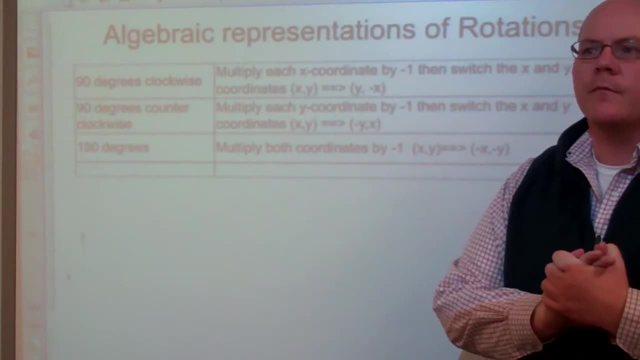 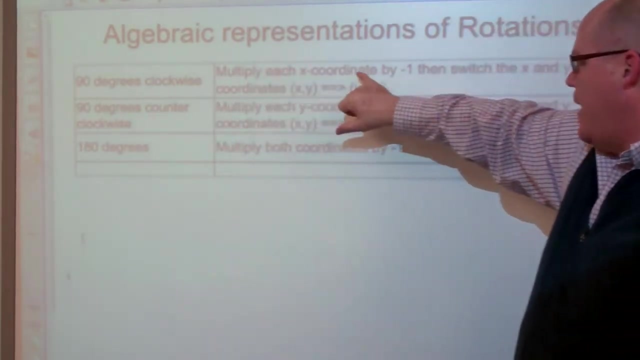 I didn't copy that down, so pause the video real quick. So when we do 90 degrees, what we do is we multiply each of the x-coordinates times negative 1, and then we switch the x and the y-coordinates. 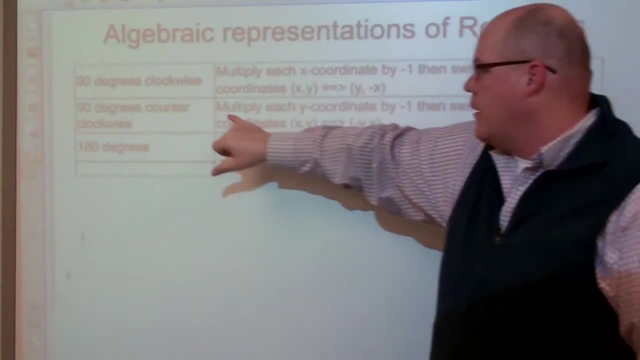 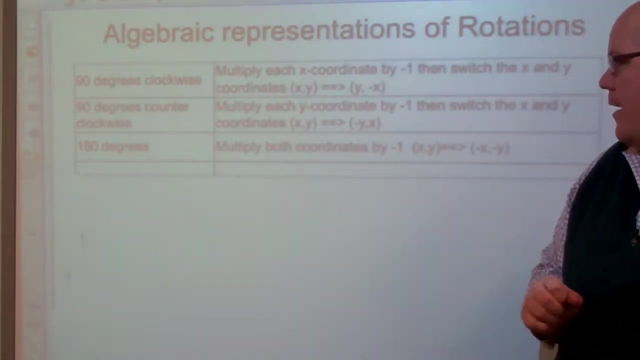 So xy becomes y negative x. Counterclockwise, we multiply the y times negative 1, and then switch to x and y. So xy becomes negative yx For 180, we're going to multiply both of the coordinates by negative 1.. 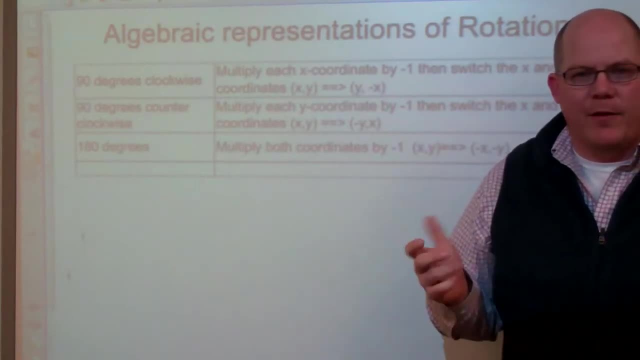 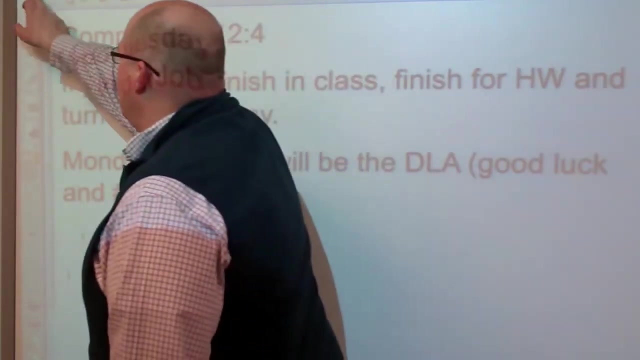 So xy becomes negative x, negative y. We're not flipping the order when we do 180.. So we're keeping them in the same order. So last thing we're doing here, guys, is I want you to go ahead and draw the table. 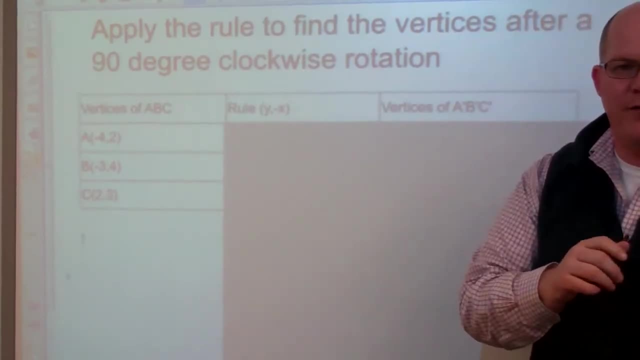 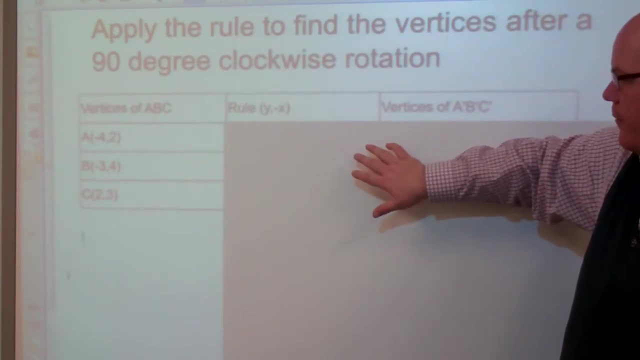 And then let's pause the video so that you guys have an opportunity to practice and complete the rest of the table. Awesome. Now that we've done that, let's go ahead and complete our table. So we have vertices of ABC. So let's see what we're doing here. 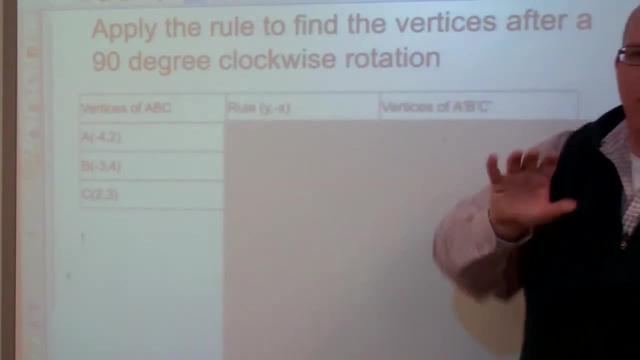 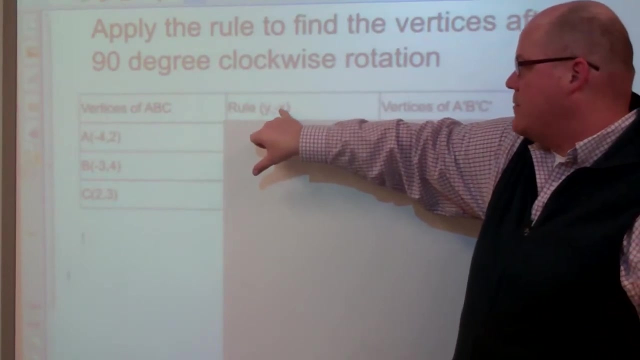 We're going 90 degrees clockwise rotation. I hope you guys realize that before you fill out the table. So I want to follow the rule, as I'm switching the y and multiplying the x times negative 1, and then switching the y and the x.